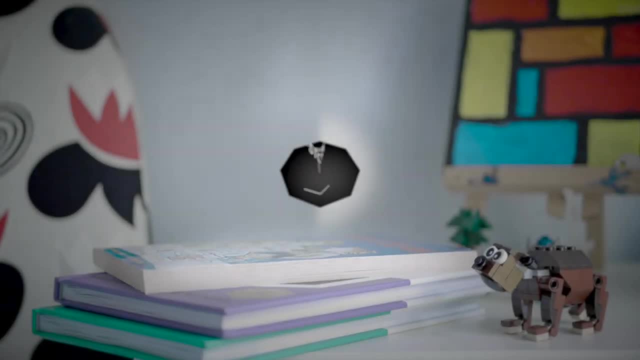 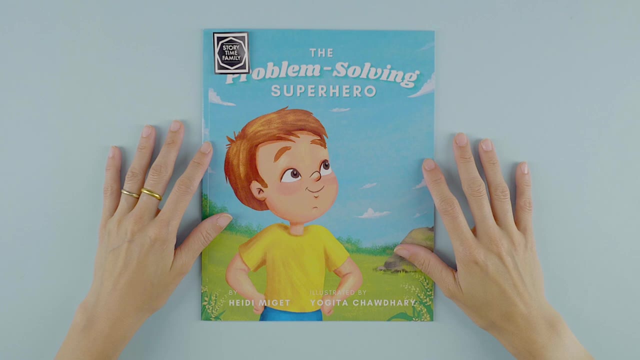 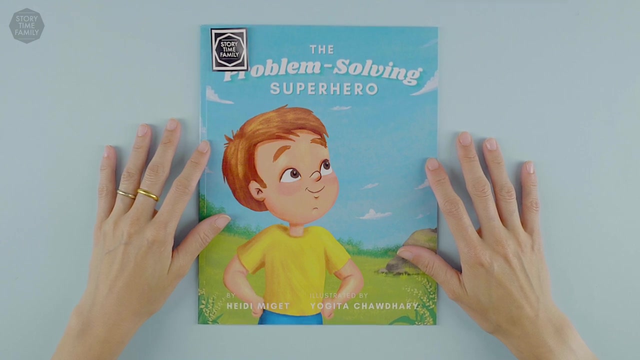 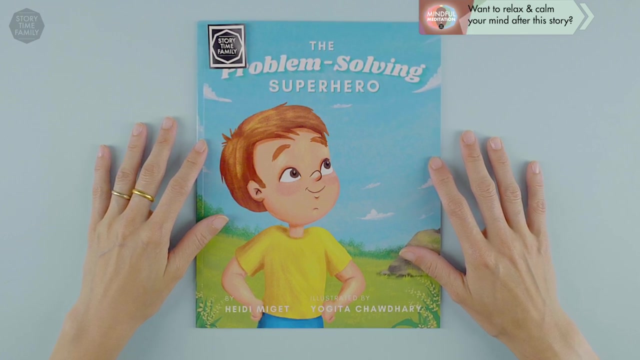 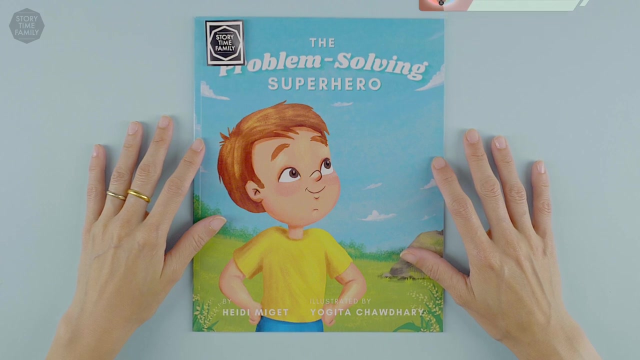 Hi everyone, welcome back to the Storytime family. How are you today? Is it nice and sunny where you are? Are you keeping warm or are you keeping cool, like I am? It's summer here and it's super hot today. I am trying to keep cool indoors and reading a book with you. Thank you so much for 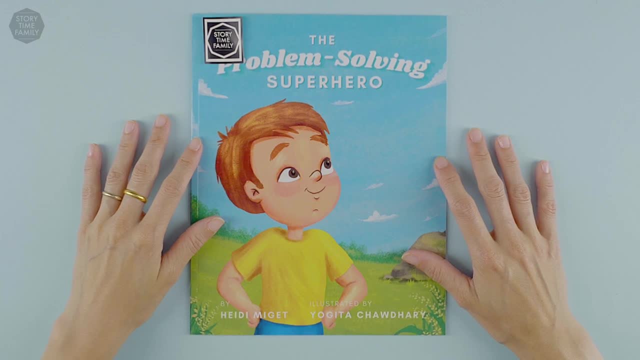 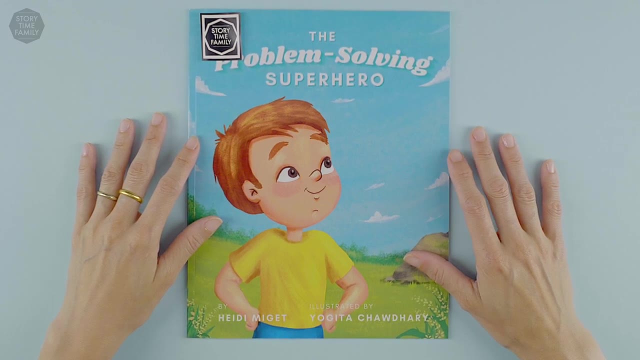 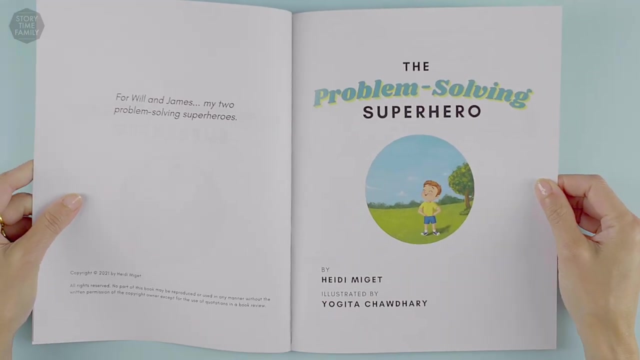 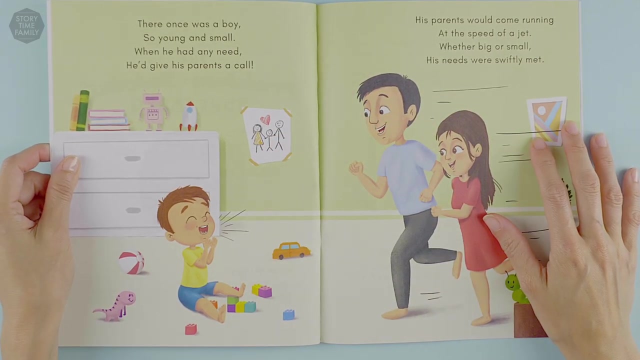 sitting down and taking the time to read with me. Today we have The Problem-Solving Superhero by Heidi Miget. Let's have a look. The Problem-Solving Superhero. There was once a boy so young and small When he had any need, he'd give his parents a call. 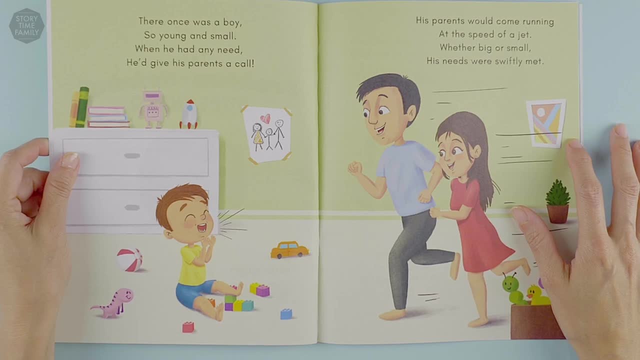 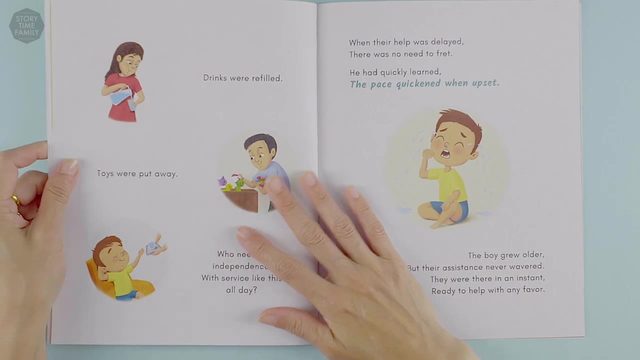 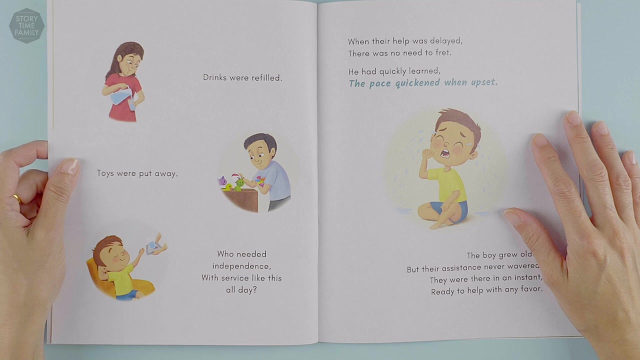 His parents would come running at the speed of a jet. Whether big or small, his needs were swiftly met. Drinks were refilled, toys were put away. Who needed independence with service like this all day? When their help was delayed, they would come running. 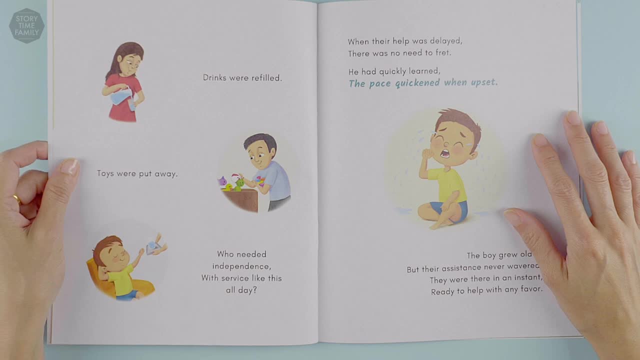 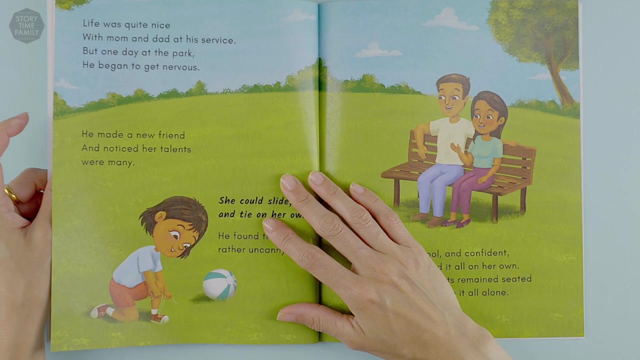 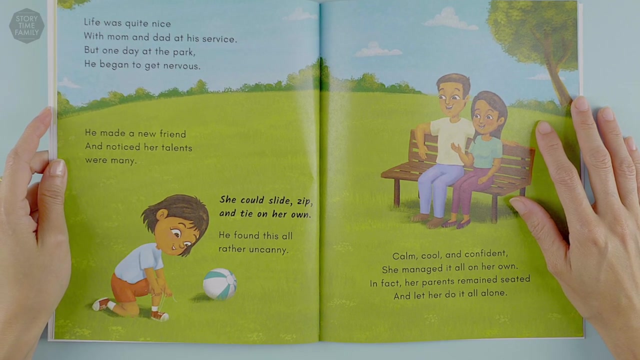 There was no need to fret. He had quickly learned. the pace quickened when upset. The boy grew older. but their assistants never wavered. They were there in an instant, ready to help with any favor. Life was quite nice with mom and dad at his service, but one day, at the park, he began to 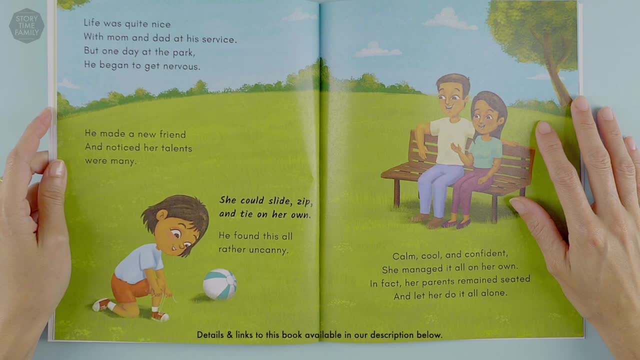 get nervous. He made a new friend and noticed her talents were manly. She could slide, zip and tie on her own. He found all this rather uncanny: Calm, cool and confident. she managed it all on her own. 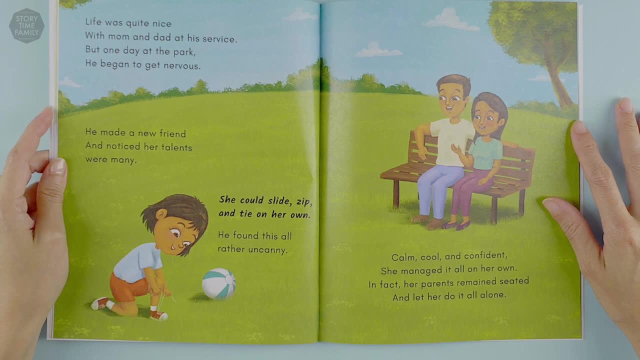 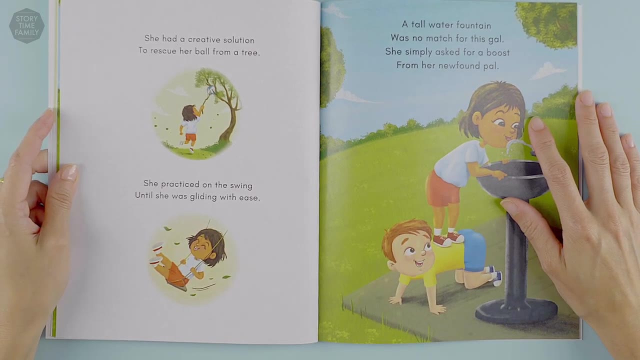 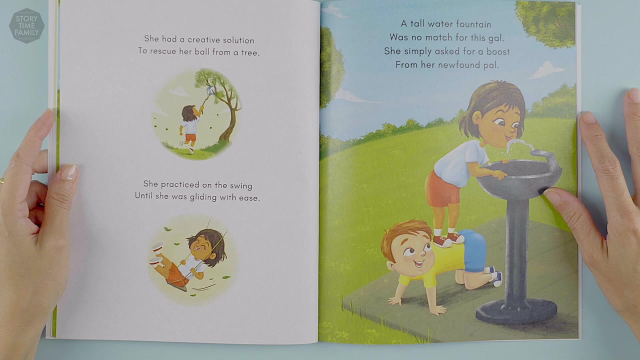 In fact, her parents remained seated and let her do it all alone. She had a creative solution to rescue her ball from a tree. She practiced on the swing until she was gliding with ease. a tall water fountain was no match for this gal. she simply asked for a boost from her newfound pal. 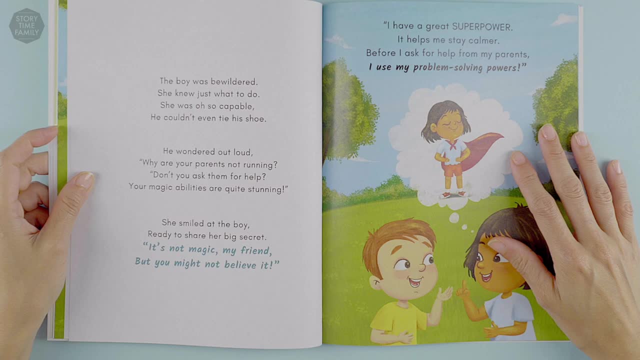 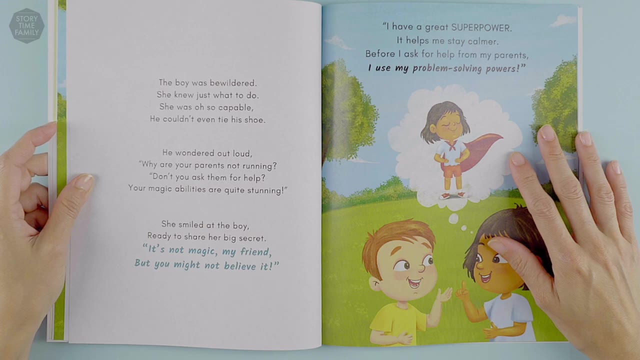 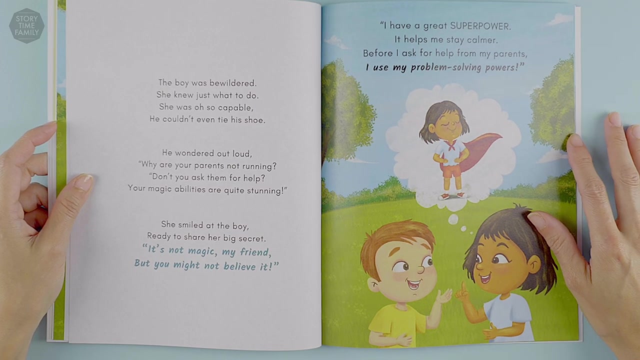 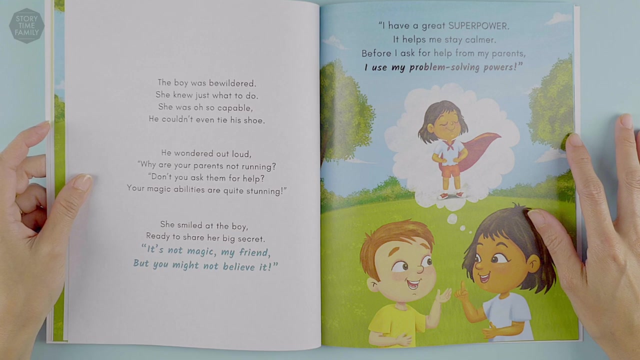 the boy was bewildered. she knew just what to do. she was oh so capable. he couldn't even tie his shoe. he wondered out loud: why are your parents not running? don't you ask them for help? your magic abilities are quite stunning. she smiled at a boy ready to share her big secret. it's not magic. my 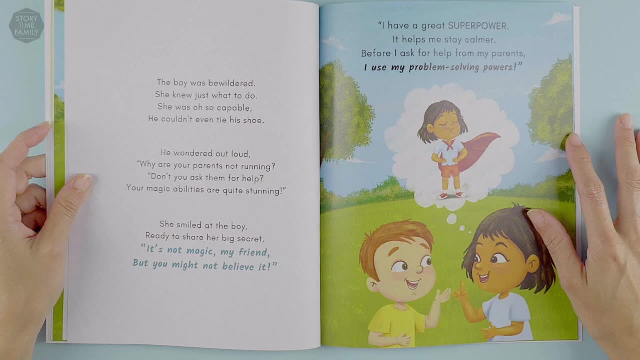 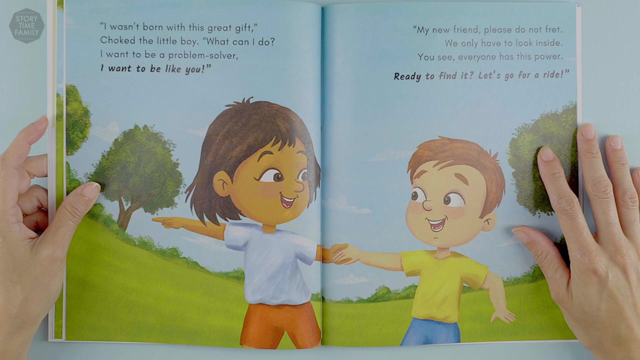 friend. but you might not believe it, i have a great superpower. it helps me stay calmer before i ask for help from my parents. i use my problem solving powers. i wasn't born with this great gift. choked the little boy. what can i do? i want to be a 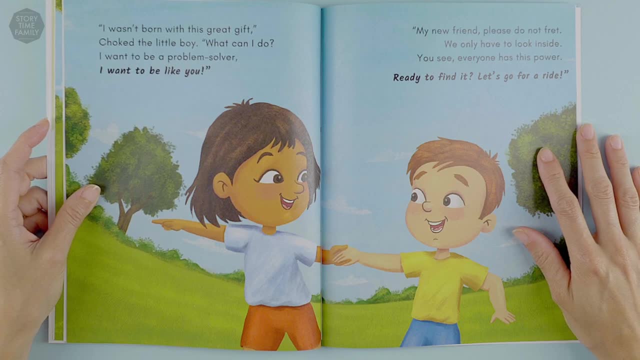 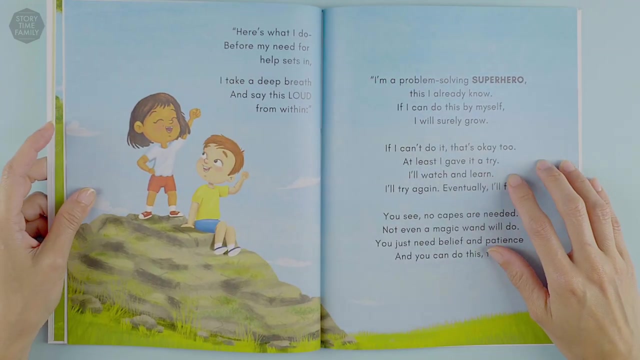 problem solver. i want to be like you, my new friend. please do not fret. we only have to look inside. you see, everyone has this power, ready to find it. let's go for a ride. here's what i do. before my need for help sets in, i take a deep breath and say this out loud from: 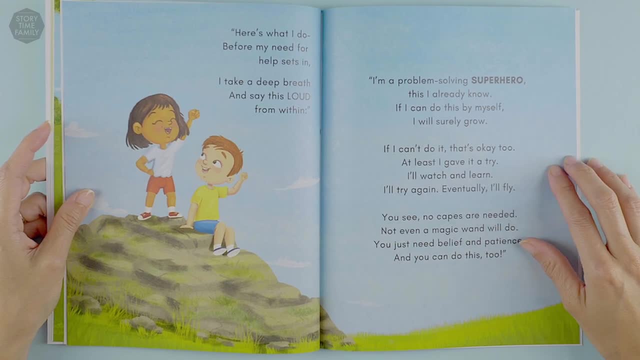 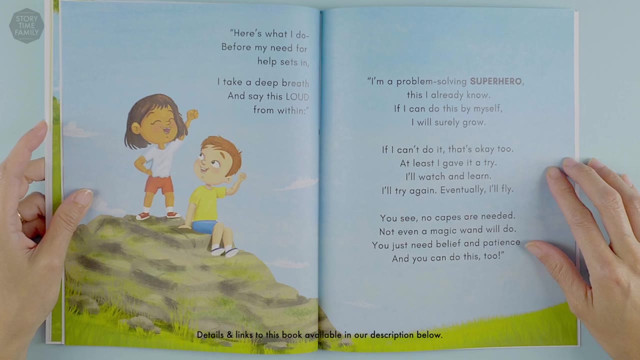 within. i'm a problem solving superhero. this i already know. if i can do this, i'm a problem solver. i want to be like you, my new friend. please do not fret. we only have to look inside, you see. no capes are needed. not even a magic wand will do. you will need belief and patience. 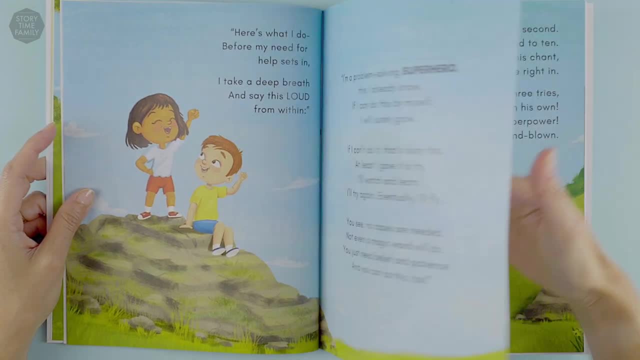 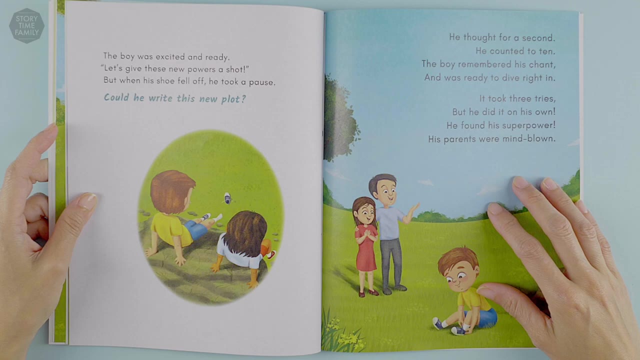 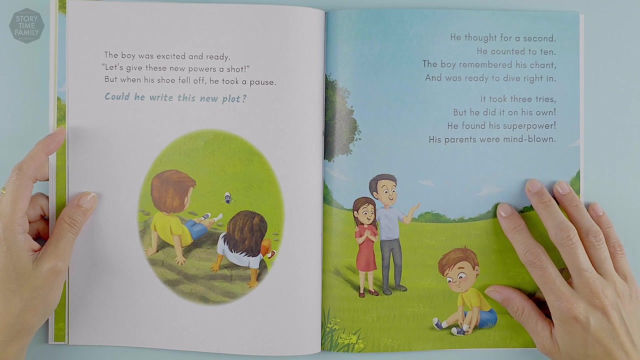 and you can do this too. the boy was excited and ready. let's give this new powers a shot. but when his shoe fell off, he took a pause. could he write this new plot? he thought for a second. he counted to 10. the boy remembered his chant and was ready to dive right in. it took three tries. 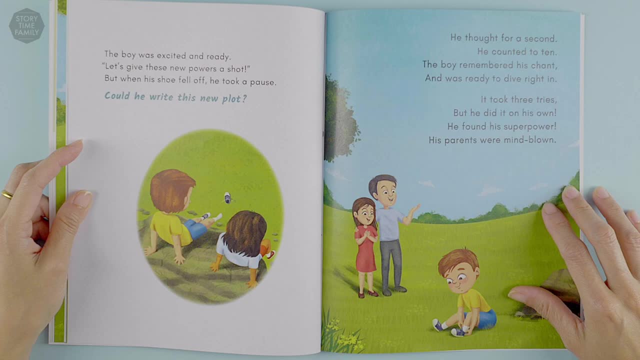 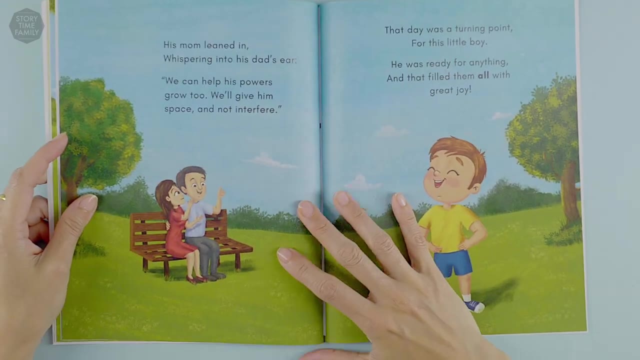 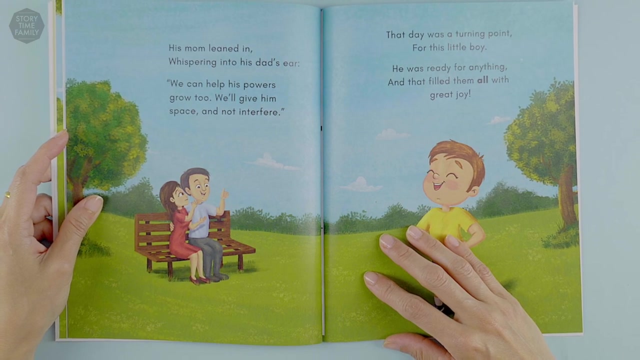 but he did it on his own. he found his superpower. his parents were mind blown. his mom leaned in, whispering into his dad's ear: we can help his powers grow too. we'll give him space and not interfere. that day was a turning point for this little boy.